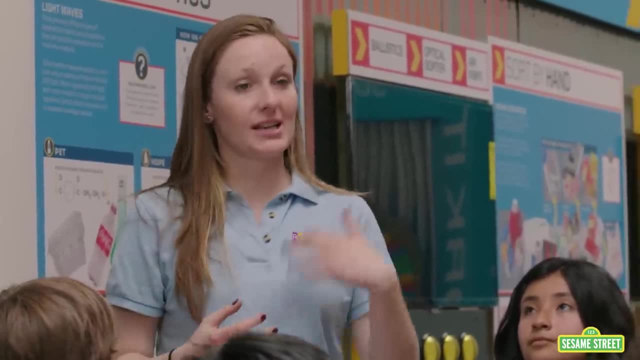 Well, trash. when you put it in the recycling bin, it's a waste. When you put something in the trash, it's gonna get put on a truck and get sent to a landfill or an incinerator and it's never gonna be used again. 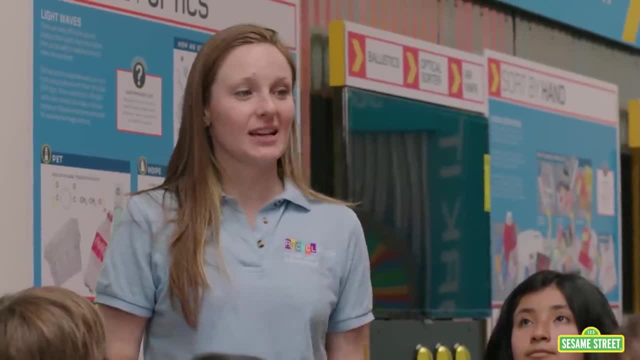 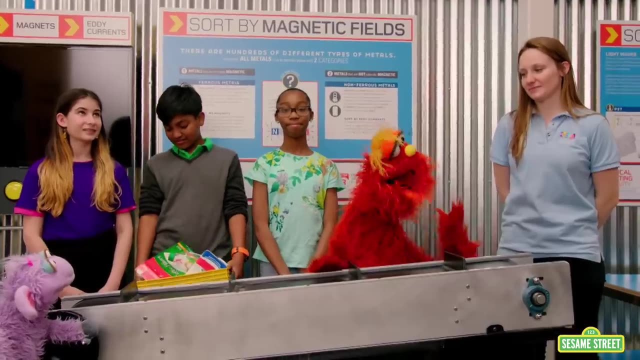 Aw, poor trash. But if you put something in the recycling bin, it comes to our recycling facility, where we'll be able to make it into a new product that can be used again by someone else, Woo-hoo, Yeah. So, Aideen, what is this station? 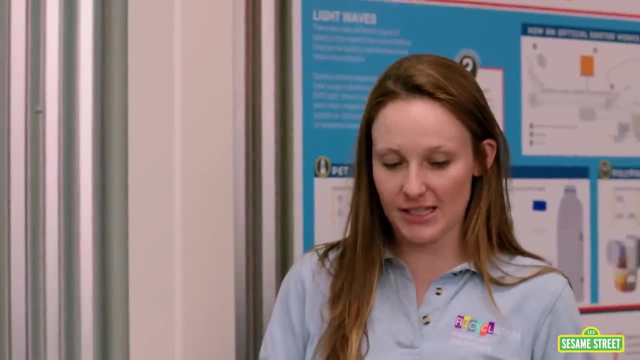 Well, this is a small version of a magnet that we have out in our recycling facility. So we put all of our recyclables onto the conveyor belt and then, when it gets to the end of the line, the magnet finds the things that have metal in it. 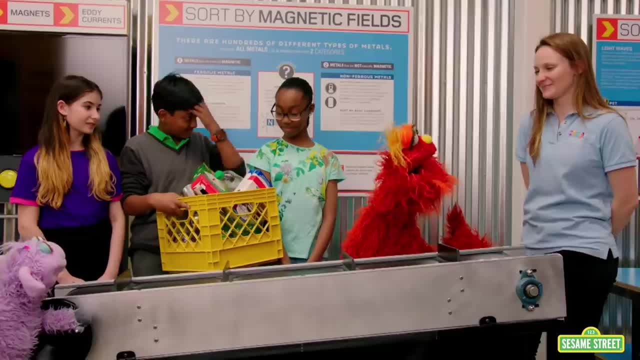 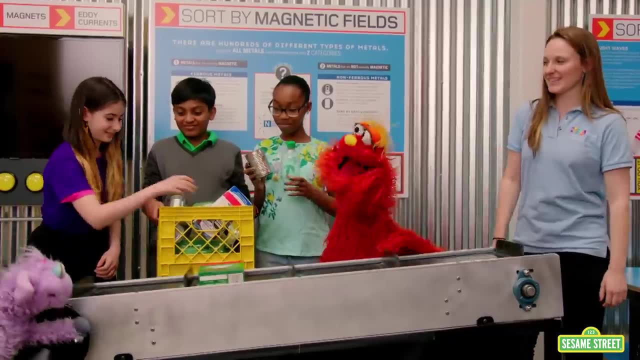 and it puts it into one bin and everything else will go into this other bin. Oh boy, Can we do it now? Yeah, we can do it now. Ready Ovejita Lista, Let's load it up. 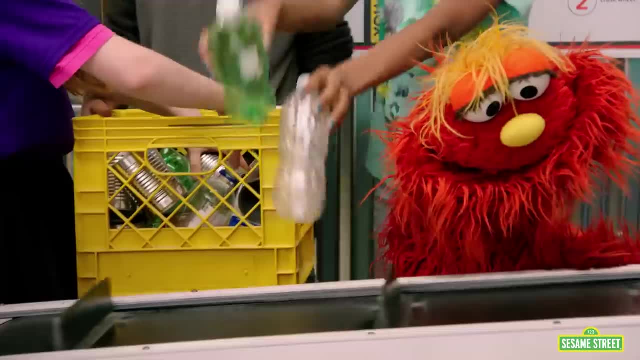 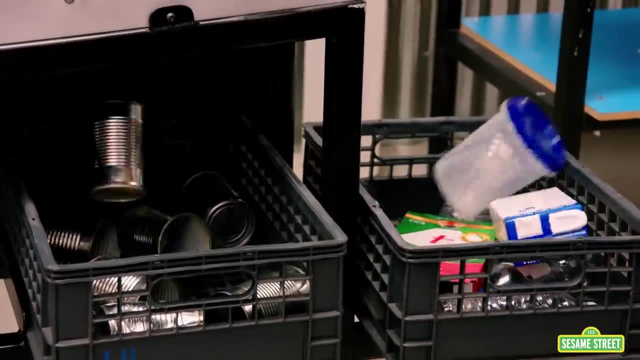 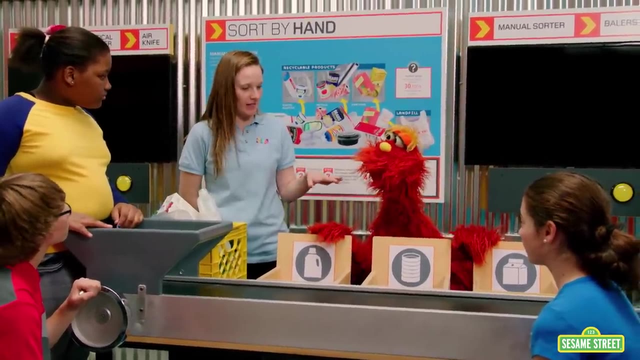 Watch the metal get sorted. Look, It's sorting the metal from the man metal. Ooh, Hey, Aideen, what happens at this station? So at this station we're gonna be sorting by hand. Keshay's gonna load on the recyclables. 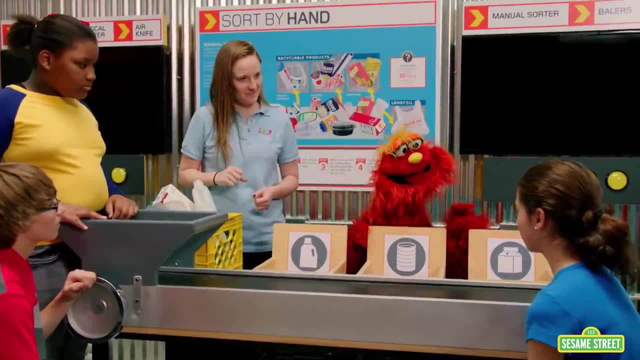 Yeah, Keegan's gonna turn the conveyor belt. Okay, the belt's gonna go. and then what's Emma gonna do? She's gonna sort out all the recyclable items, but if they end up at the end, they're gonna have to go to a landfill. 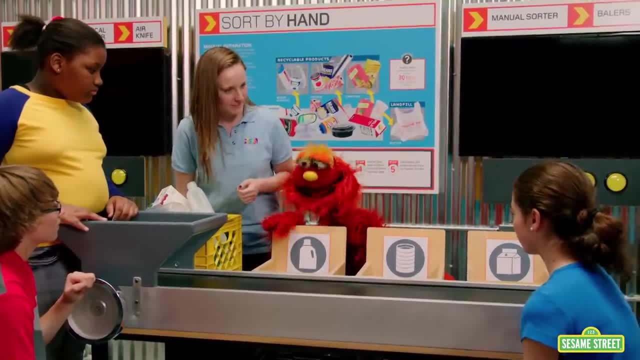 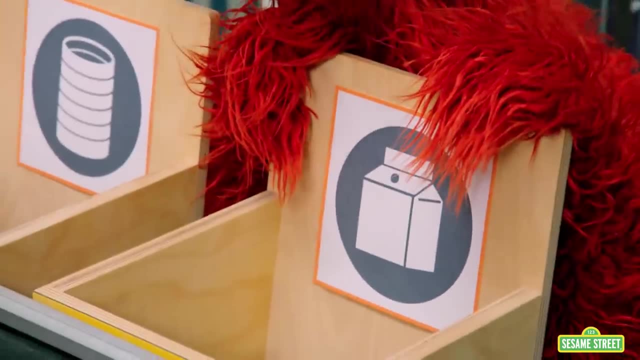 Oh, what goes in this bin? This one is plastic. Okay, Emma, this is plastic. And then what goes in this bin? Metal, Metal. You got that, Emma. And then what goes in this one? Cartons, Cartons. 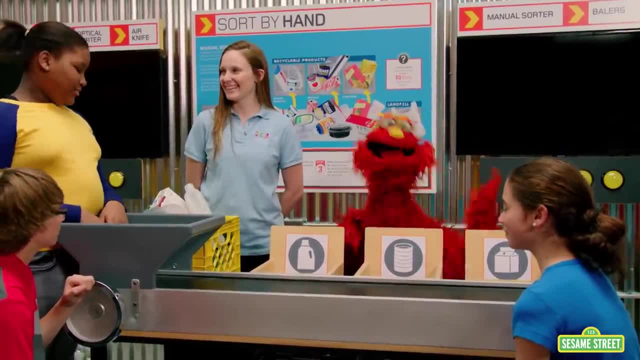 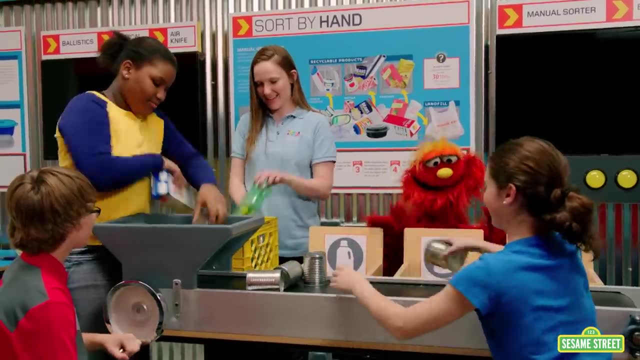 Emma, you ready, All ready, Guys, you ready, Ready? Let the sorting begin. Okay, let's go. That goes in. Come on Emma. Okay, sir, Going in the plastic. Okay, Come on Emma. 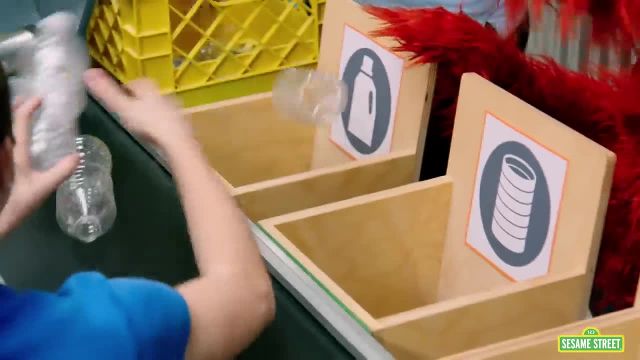 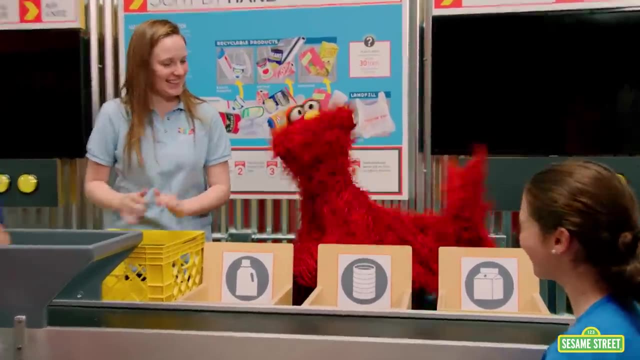 Make it go faster, Keegan, Make it a challenge. Metal plastics, Metal, metal plastic. Whoo Ha ha ha. We did it, We sorted everything. Hey Dean, what happens here? This is the tipping floor where the recyclables 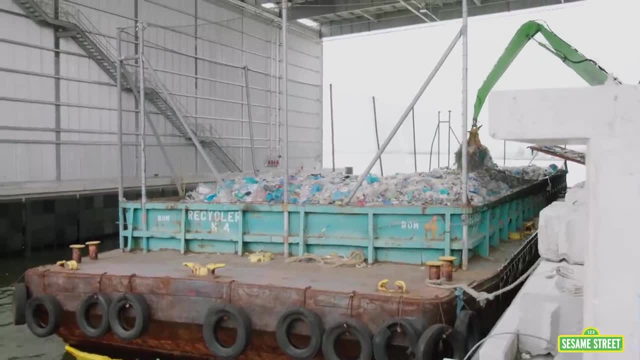 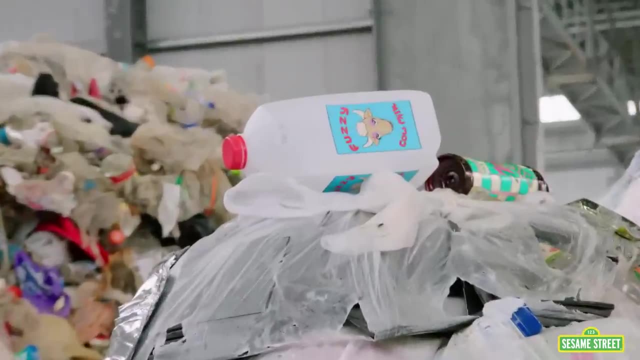 come in on trucks or on big boats called barges. Whoa, This is a lot of recyclables. Ha ha, Whoo Whoo. Look, It's my milk jug. Hey Dean, what's gonna happen to my milk jug now? 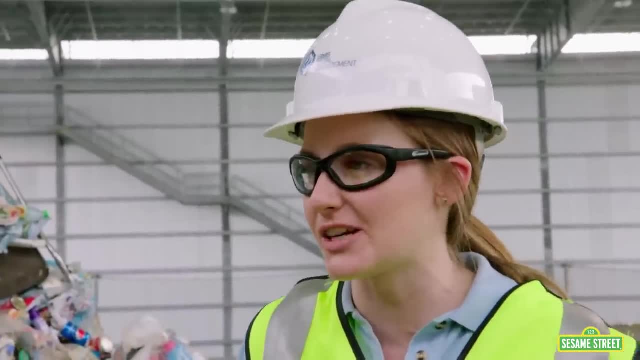 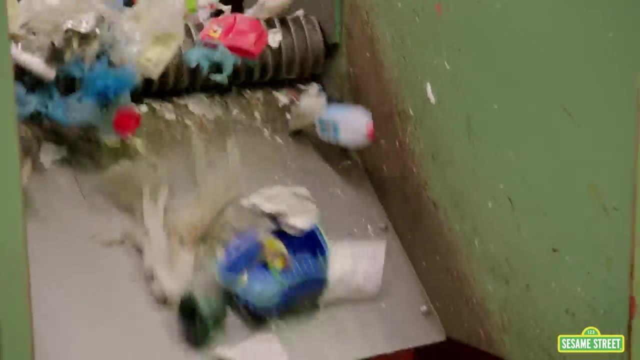 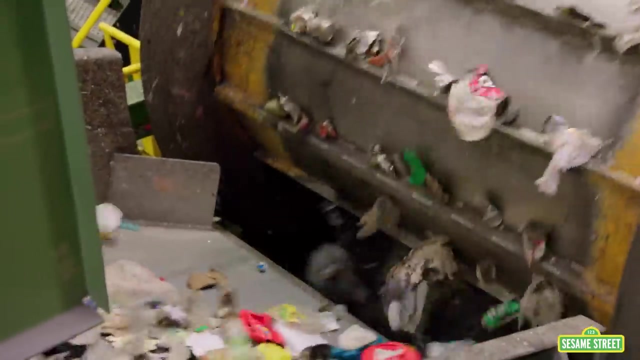 Your bottle's gonna go into the recycling sorting and it's gonna separate with other milk jugs. Whoa, Come on, Let's check it out. Wow, Look at all the metal getting picked up by the magnet. Whoo, Look. 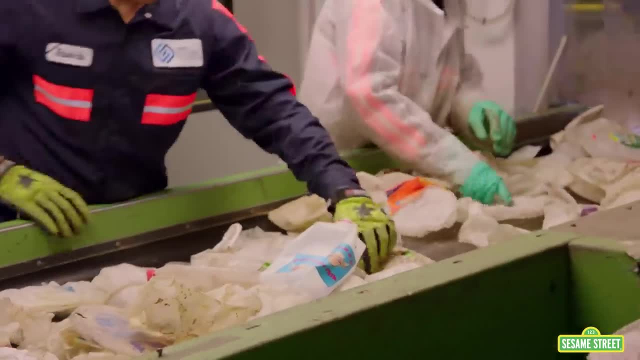 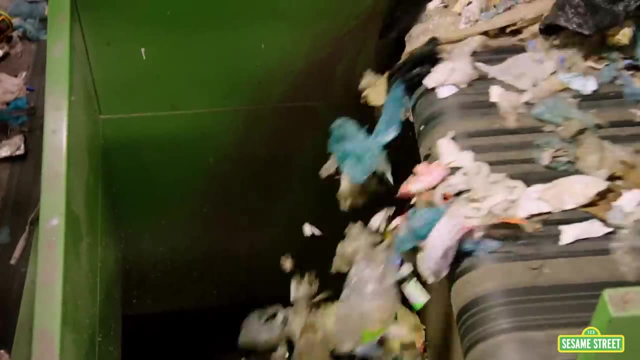 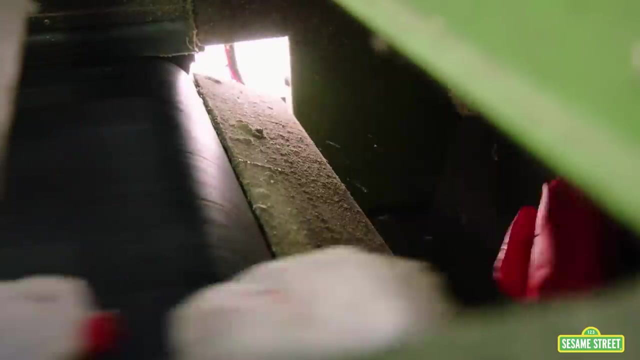 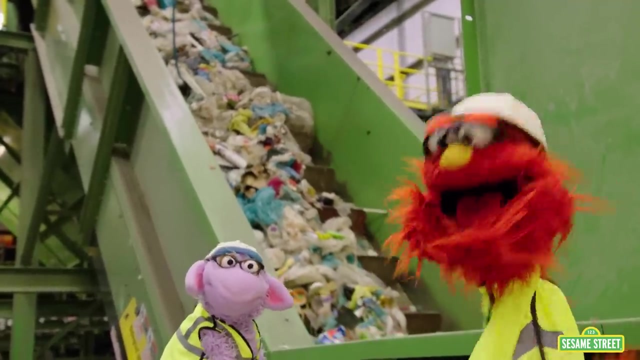 I'm sorting everything by hand. My milk jug, Uh-oh, Uh-oh, Let's try it again. My milk jug, I got it. My milk jug, My milk jug. Sorted glass- Whoa, that's a lot of recycle. 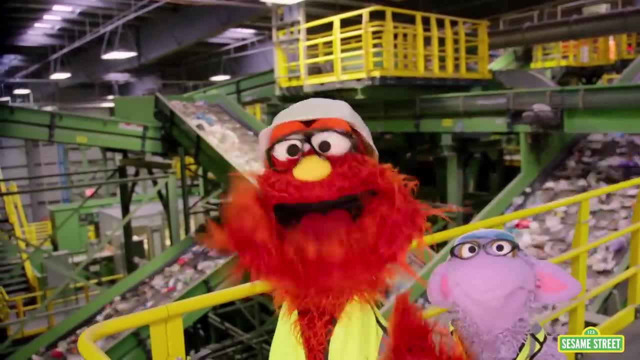 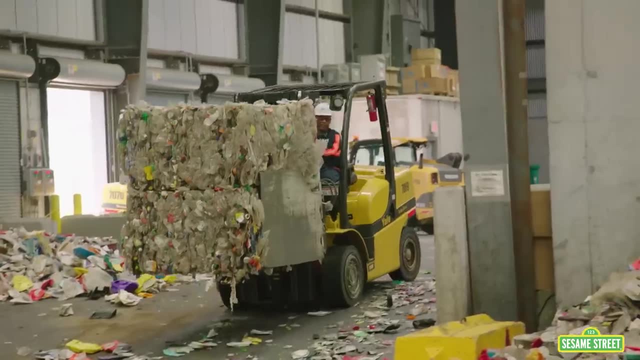 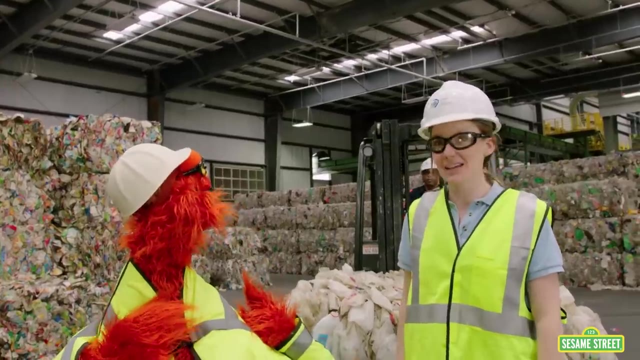 Metals, plastic, glass, So many types. Oh, Lid things to sort. Aideen, what is all this stuff in here? These are all our sorted recyclables. They're all sorted. Yep, Wow, Hey, look, there's my milk jug. 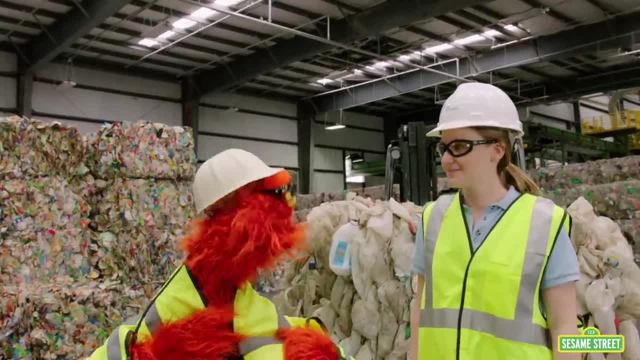 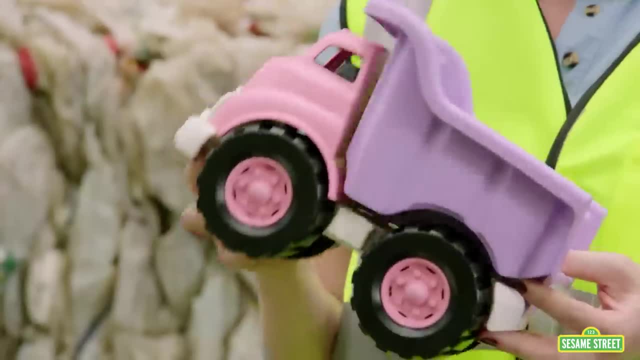 Aideen. what kind of things can all this stuff be recycled into? Well, it can be recycled into all kinds of things. For instance, your milk jug could even be recycled back into a toy. Whoa, This is made from recycled plastic. Yeah, 100 percent. 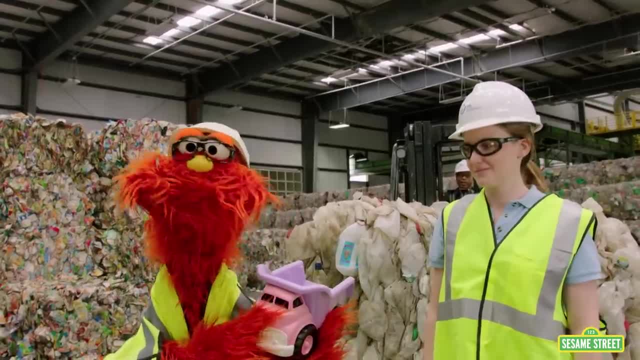 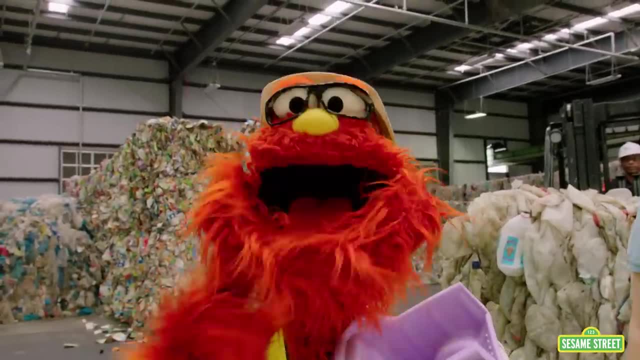 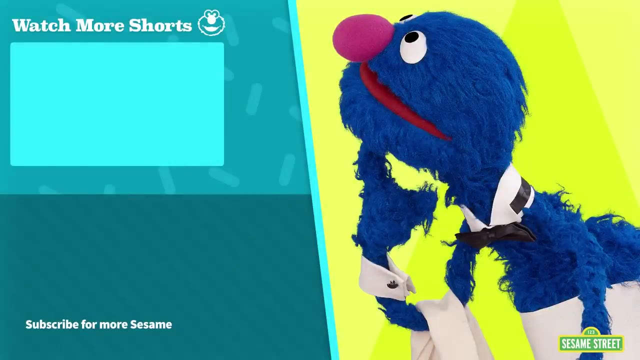 My milk jug may become a plastic cool toy truck. Good luck, little milk jug. I love sorting and I love recycling. Captions by GetTranscribedcom.